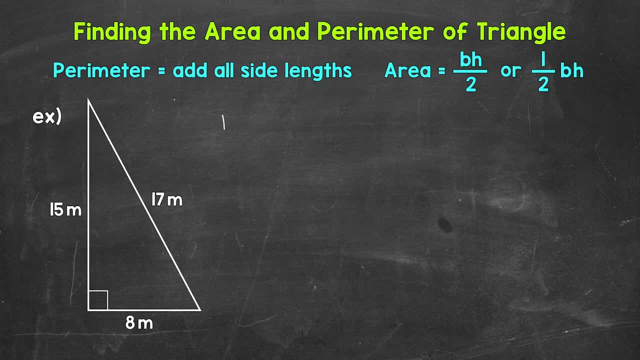 the perimeter of this right triangle. So perimeter equals. and then again for perimeter, we need to add all of these side lengths. So we have 15 meters, 17 meters and 8 meters, So 15 plus 17 plus 8.. Keep in mind, it doesn't matter what order you add the side lengths. 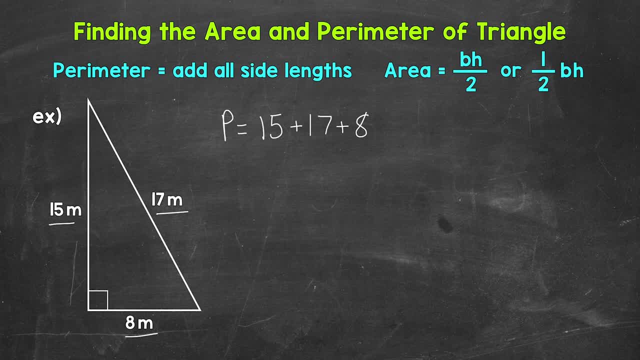 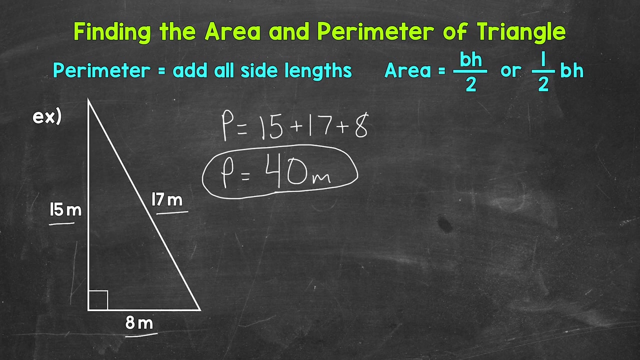 in, you'll get the correct perimeter however you do it. So let's start with 15 plus 17,. that gives us 32, plus 8 gives us 40. So the perimeter equals 40 meters. Now we can move on to finding the area of this triangle, and we can start by writing. 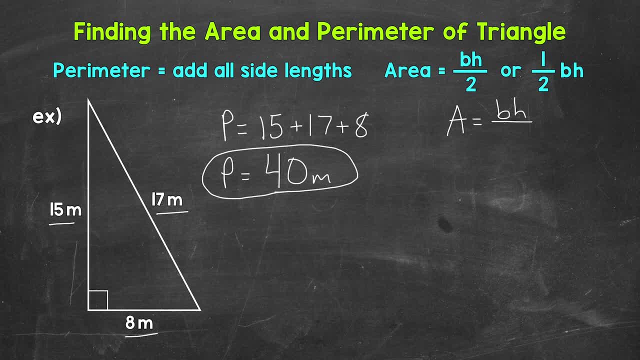 out the formula. So area equals base times height divided by two. Let's plug in the base and height. now We're going to use 8 meters for the base and then 15 meters for the height. We do not need this 17 meters in order to calculate the area. 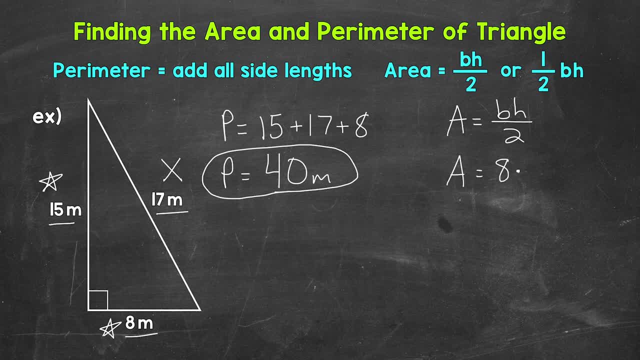 So let's plug in 8 meters for the base times 15 meters for the height divided by 2.. Now we can work through this. So let's start with 8 times 15, that gives us 120.. So we have 120 divided by 2.. 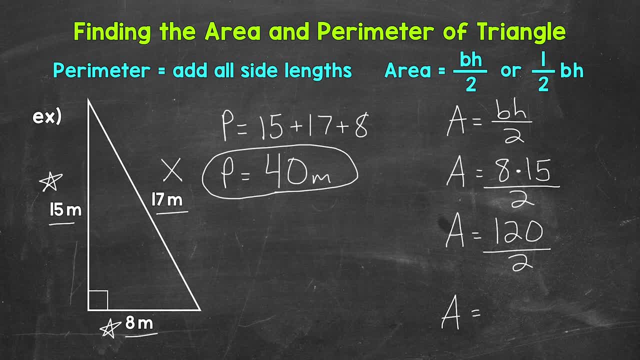 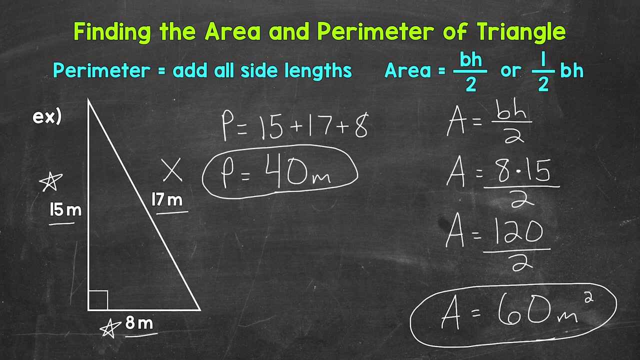 120 divided by 2 gives us a final area of 60 square meters. So for that right triangle we have a perimeter of 40 meters and an area of 60 square meters. So there you have it. There's how to find the area and perimeter of a triangle, And specifically, 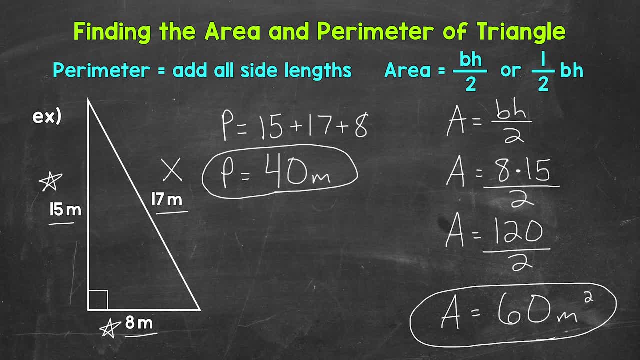 we worked with a right triangle. Just remember: for the perimeter we add all of the side lengths And then for the area of a triangle we can either use base times height divided by 2, or 1 half times height. I hope that helped. Thanks so much for watching. Until next time, peace. Subtitles by the Amaraorg community.